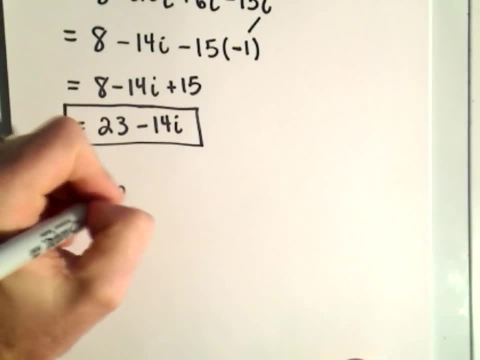 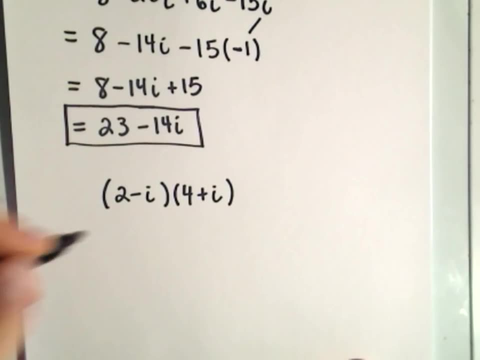 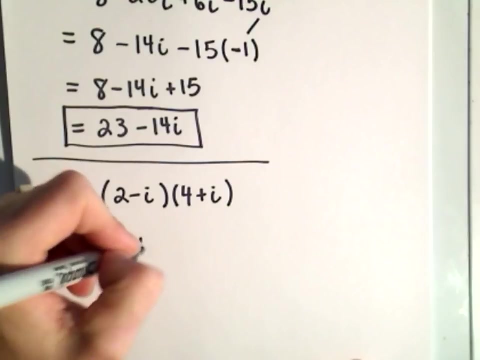 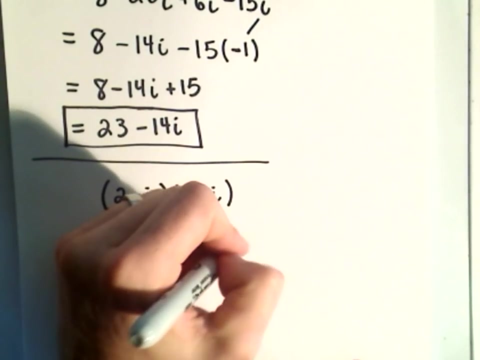 Suppose it was the number I don't know, 2 minus i, and then maybe it was 4i. Well, in this case again, we just FOIL things out: 2 and 4 is 8, 2 times i will be positive 2i. on the inside, we'll get negative 4i, and then on the outside we'll get negative. i squared. 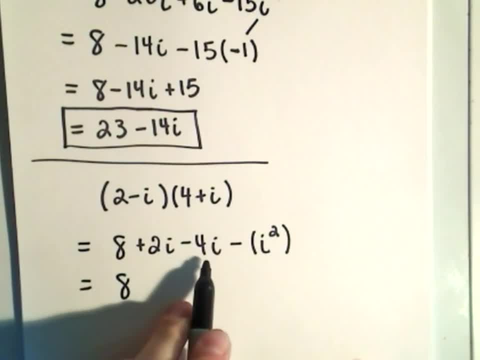 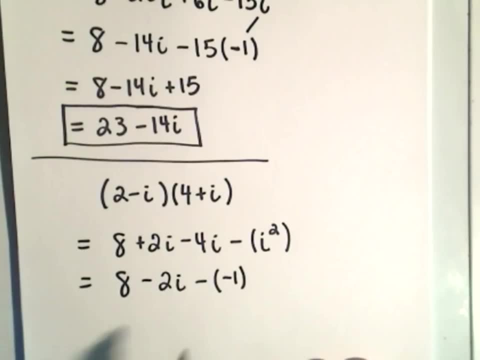 So again, this will give us 8 positive. 2 minus 4 is negative. 2i- i squared again- is negative 1, so really I'm subtracting away a negative which is a positive. so really I get 8 plus 1, which is 9 minus 2i, and that will be my solution. 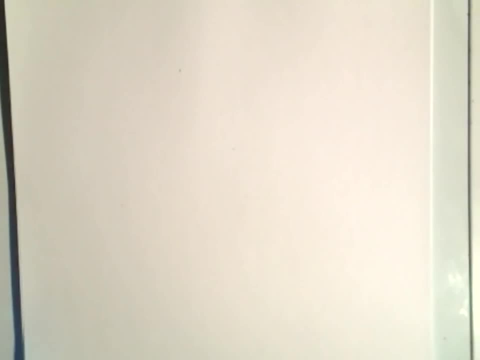 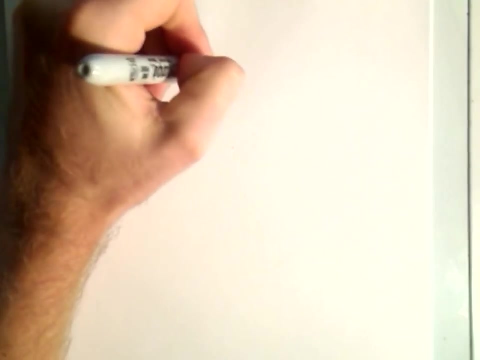 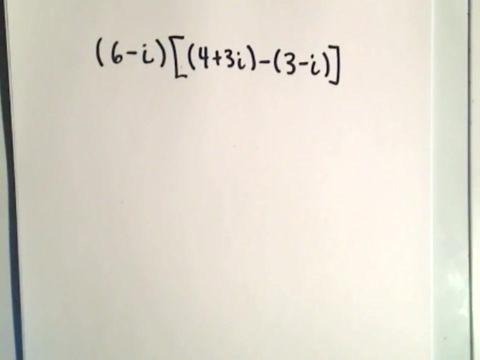 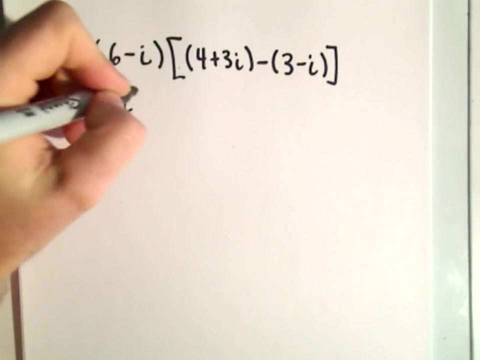 Okay, so maybe let's do one more multiplication example. Suppose it was 6 minus i, and then inside the brackets we had 4 plus i minus 3 minus i. Well, in the first case here we would want to simplify things down inside the brackets, so I would leave the 6 minus i out front alone. 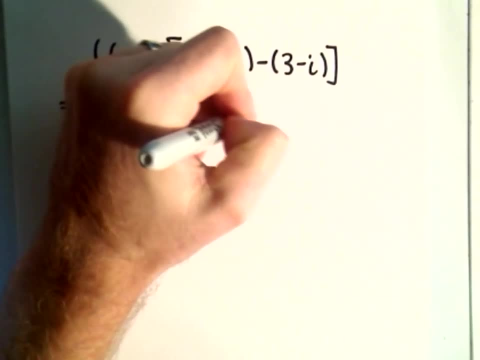 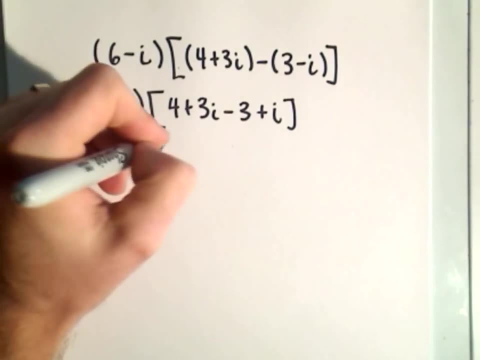 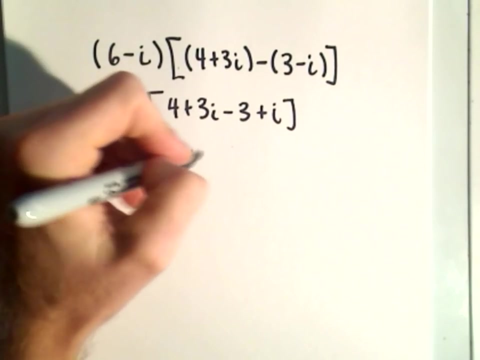 So we would have 4 plus 3i minus 3 plus i. when I distribute, so that's 6 minus i. Inside the brackets we'll get 4 minus 3, which is 1, and then we have positive 3i plus 1i, which is plus 4i. 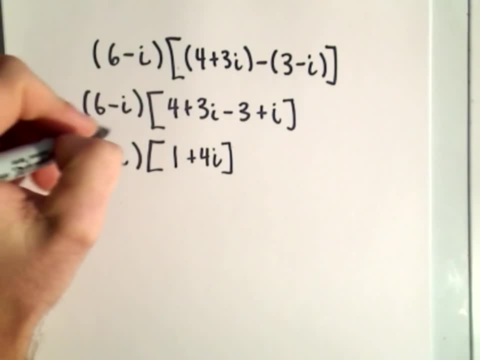 Okay, and now we'll just FOIL this out like before: 6 times 1 is 6,. 6 times positive 4i is positive 24i. on the inside we'll get minus i and then on the outside we'll get minus 4i- squared. 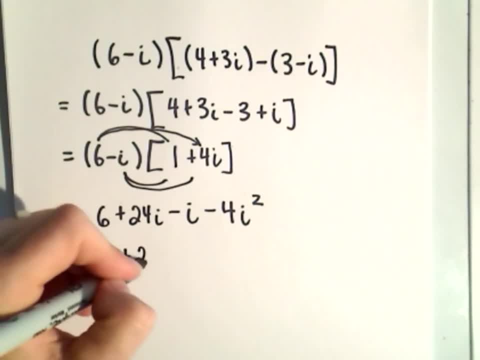 So this is 6, 24i minus i is positive 23i. i squared is negative 1, so the last term will turn into a positive 4, so we'll be left with. So we'll be left with 10 plus 23i when we combine our like terms. 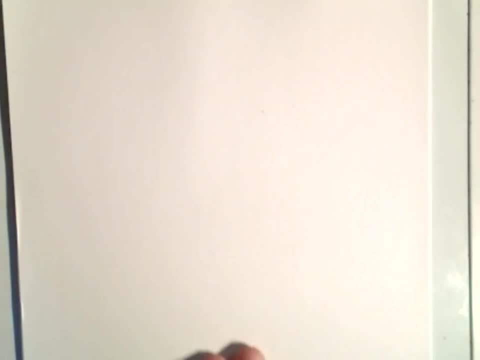 Alright, so let me talk about dividing complex numbers. So when we divide complex numbers, 5 plus 2i over 4 minus i- I should mention real quick, if we just have a complex number divided by a real number, suppose it was 8.. 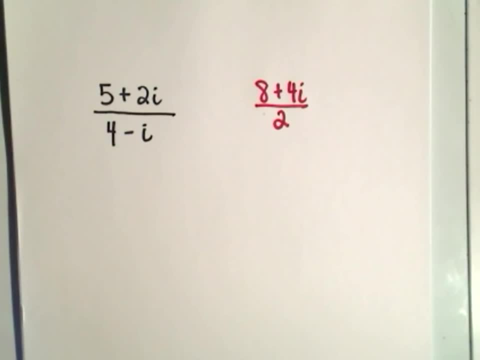 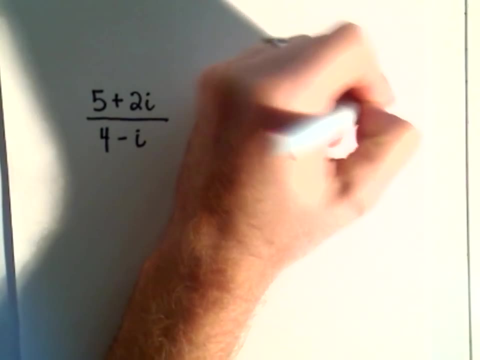 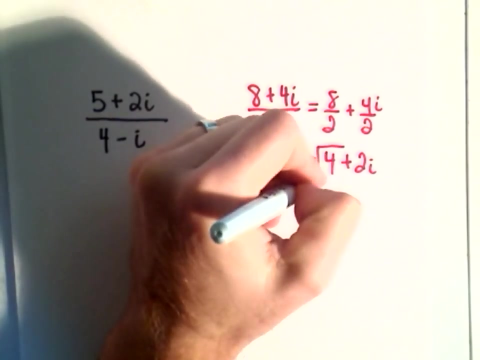 Plus 4i divided by 2, you could basically bust this up like a normal fraction and make it 8 over 2, plus 4 over 2, stick the i in there. So 8 over 2 is 4,, 4 over 2 is 2i, and that would be your solution. 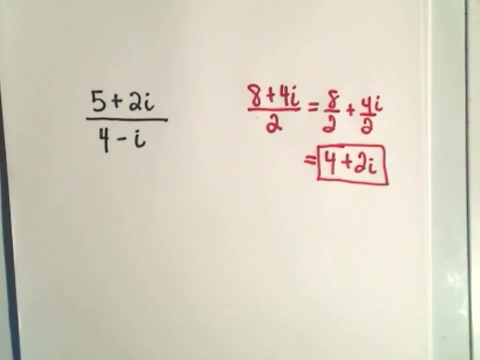 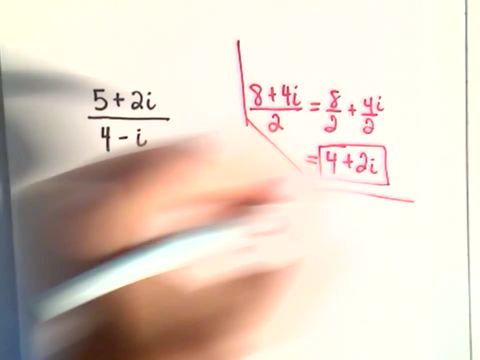 So if you're dividing by a part that just has a real number, that's all you'd have to do, Okay. but in this example there is This: 4 minus i, and what we do in the denominator: you multiply by the conjugate. 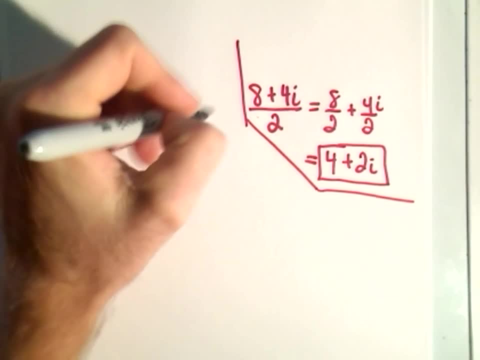 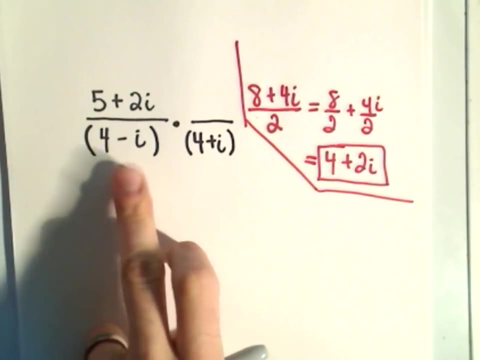 Basically, you want to try to get rid of the stuff in the bottom, So I'm going to multiply the denominator by 4 plus i, and the conjugate again is just when you leave. basically, whatever it is, you just flip the sign in the middle. 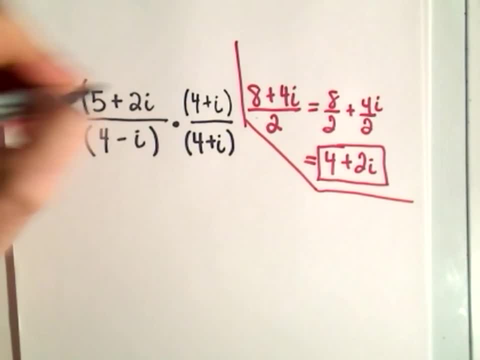 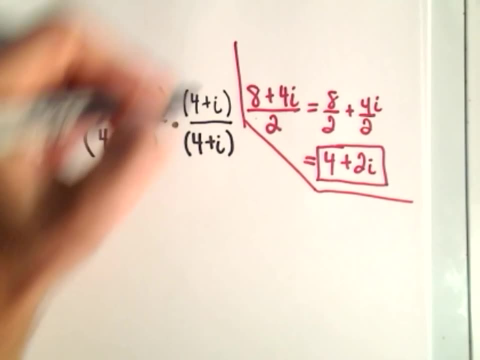 If I multiply it to the bottom, I'm going to have to multiply it to the top, And now I need to FOIL out the top, so I'll get 4 times 5, which is 20.. 5 times i is 5i. 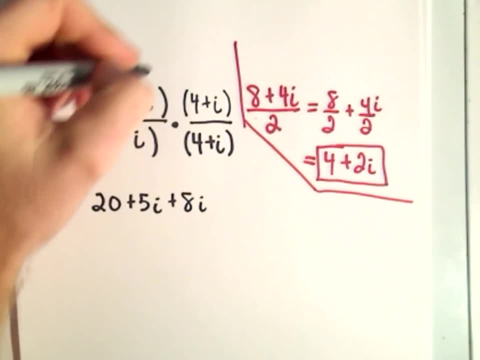 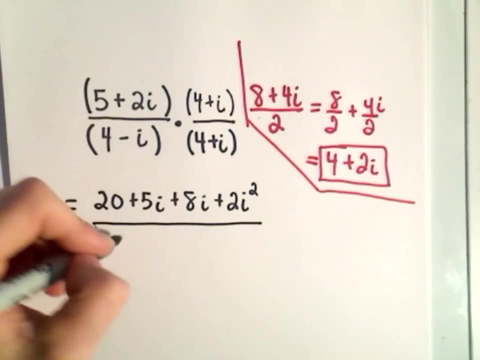 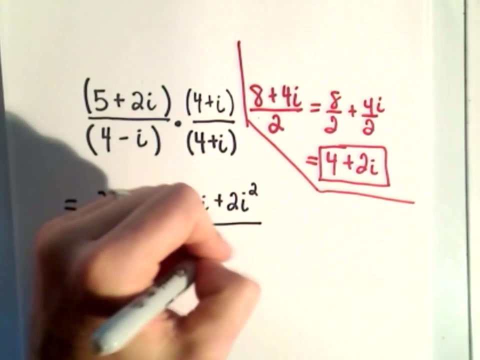 On the inside I'll get positive 8i And then on the outside I'll get positive 2i squared when I FOIL out the numerator. When I FOIL out the denominator, I'll get 16 plus 4i, minus 4i, and then I'll have a negative i squared term. 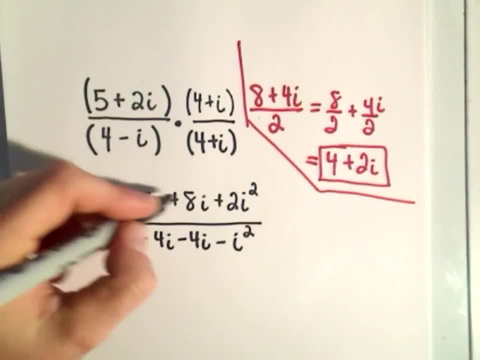 So on top, we have 20.. 5i and 8i is 13i, And then we'll have i squared, which is negative 1.. On the bottom, we have 16.. Notice: the positive 4i and the negative 4i will cancel. 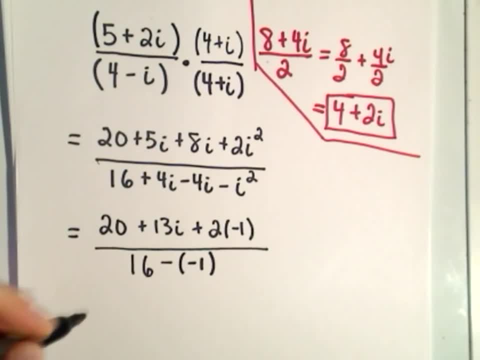 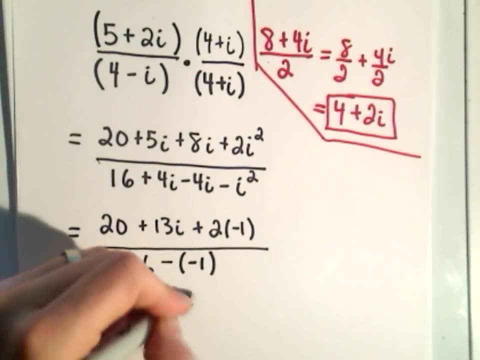 And then we have minus i squared, which is negative 1.. So on top, we're going to have 20 minus 2, or 18, plus 13i. On the bottom, we'll have 16 plus 1, or 17.. 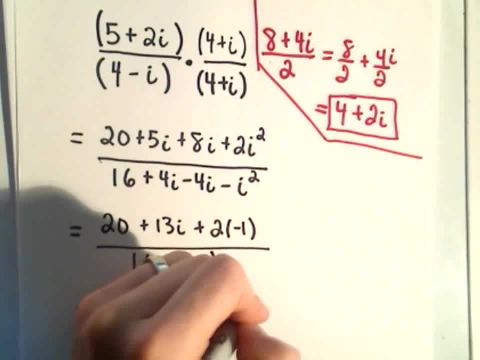 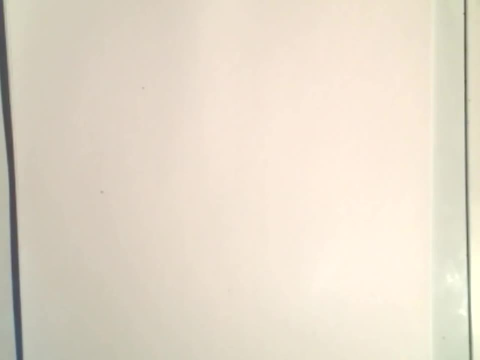 And now we can just bust this up and make it 18i, 18 over 17, plus 13i over 17,, and since that doesn't reduce, that will be our solution. So maybe let's do one more division one here.